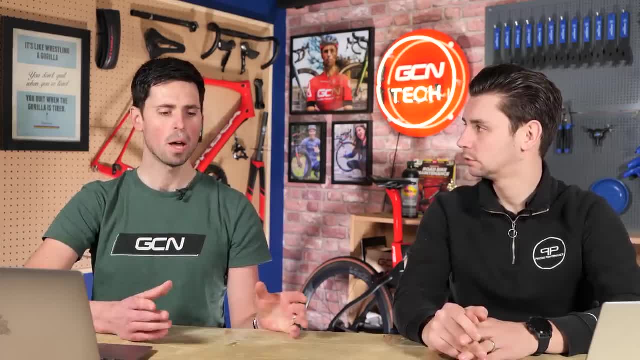 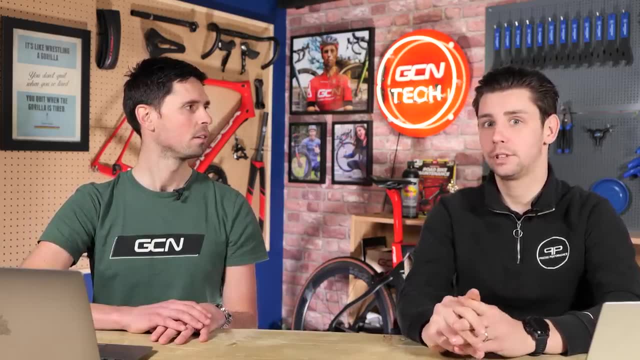 There's 170,, 172.5, and 175.. Are there options that are longer or shorter than that? in the extreme, shall we say Absolutely yes. I've seen crank lengths down to 155 millimeters and- Super short. 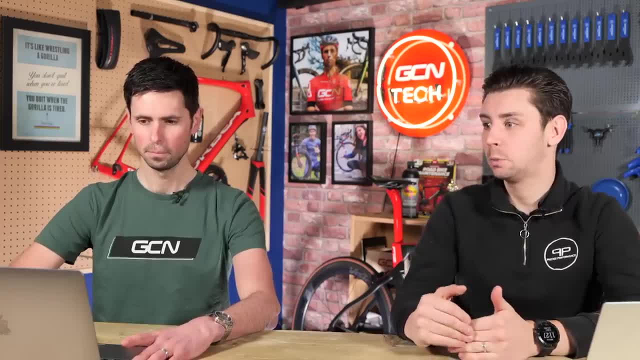 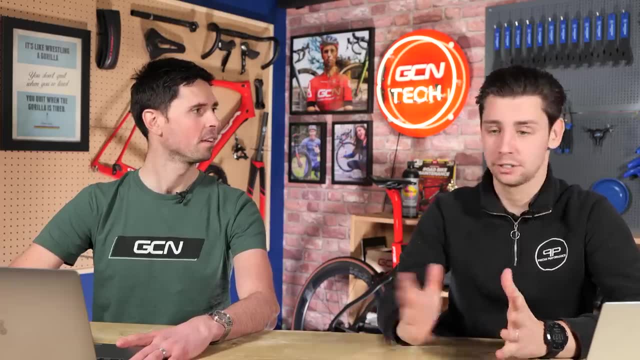 Super short. yes, You also get them 165, 180.. I don't know if they still actually make it, but there was a 177.5.. Oh, real specific, Real specific. I don't know why they even needed to do that, but yes, it's there. 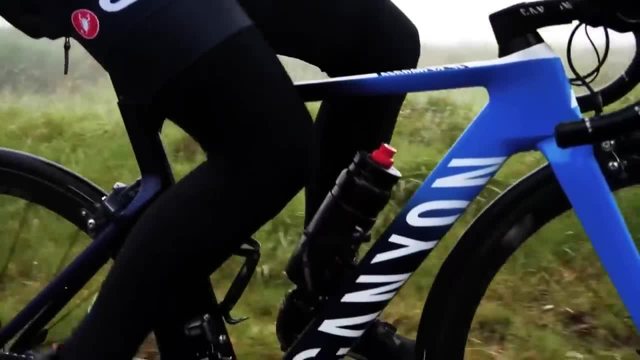 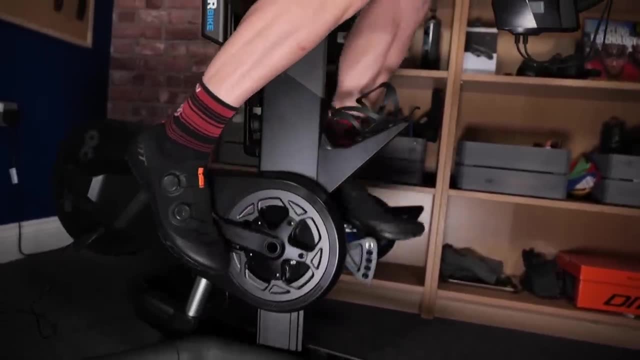 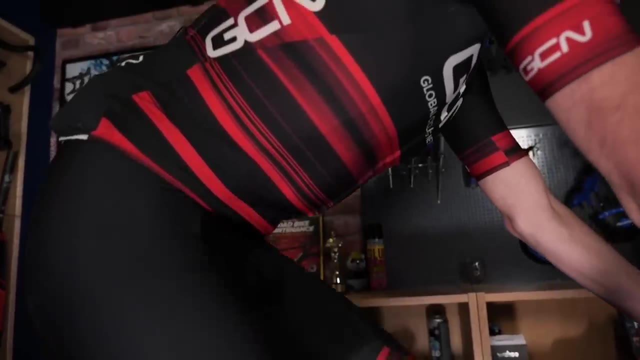 In general terms, how does the crank length affect the range of movement that you have? We're referring to hips mostly- Yes, Most of the time the rider's hips. if they're a little bit limited or they can't sort of like- If you imagine trying to touch your toes, you can't close your hips up too much on a. 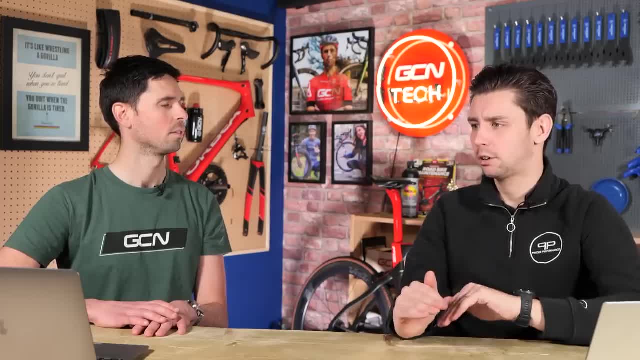 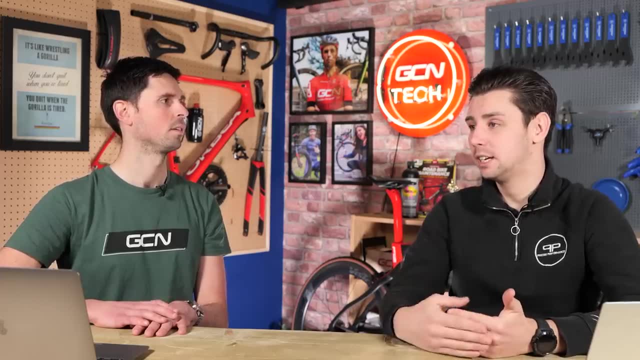 very, very simple format. We might need a shorter crank to allow the hip to stay open when they're actually pedaling the bike, which then reduces the risk of injury, improves the efficiency and, in turn, if you're more comfortable, you're going to be more efficient anyway. 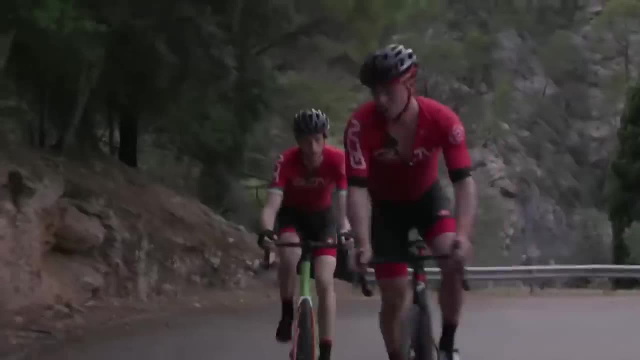 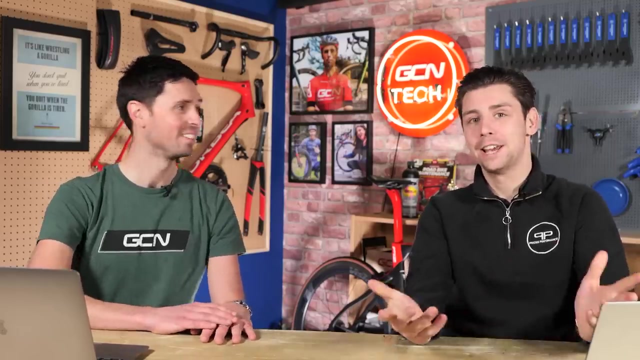 How- How are you going to know that what is installed on your bike is actually correct? How do you know that it's right at first? Well, you may not, You might, Oh. wow, It's kind of hard to know what is. 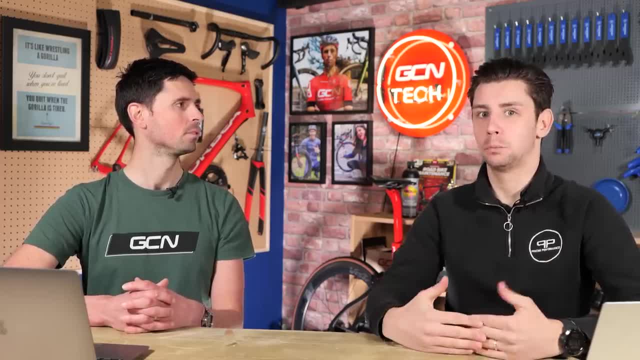 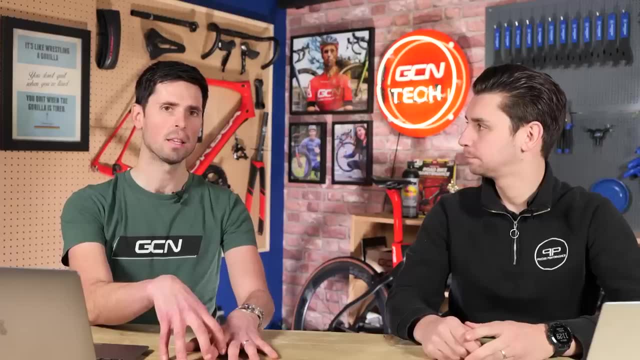 correct unless you do go through the relevant steps of understanding what your body's limitations are and why you may benefit from a shorter crank. A pretty clear indicator that you need to make a change or something could be off is if you've got an injury or you're finding 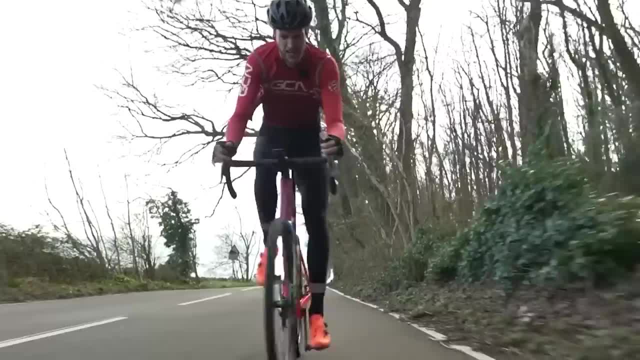 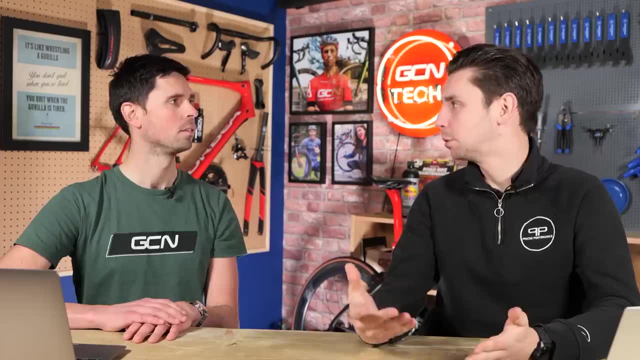 that you've got a persistent niggle- Yes, A niggle- in your knee or your hip, or you're finding that your movement's limited on the bike. Is that all right? Okay, The common things that you may find if your crank length is wrong or potentially not optimal is some knee pain, some hip pain. 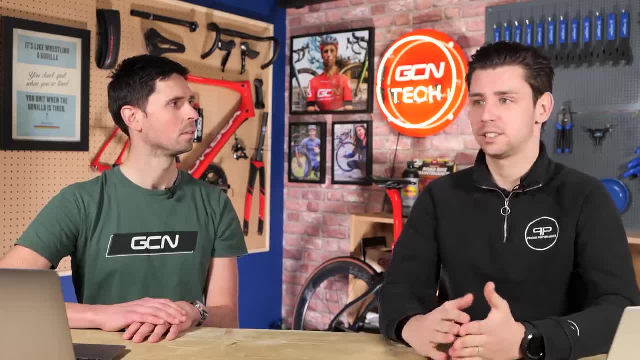 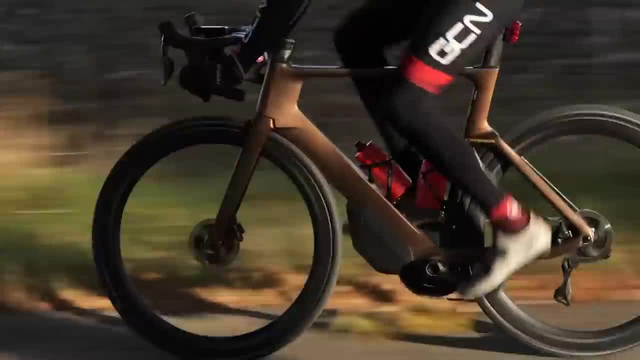 some pedaling alignment issues. Potentially, your pedal stroke isn't as smooth. Granted, you might need to try a different crank length to actually know that difference. Do you reckon, if I don't know if I went and stole Ollie's bike, change his crank? 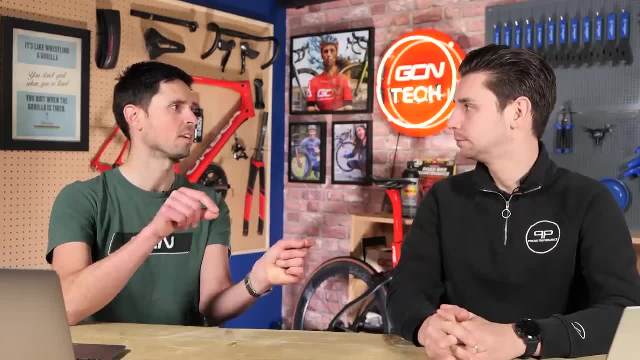 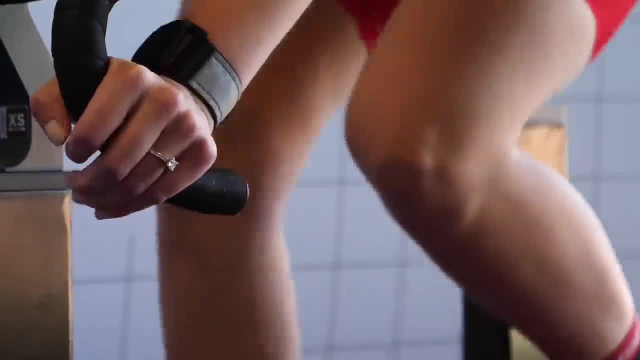 length from, well, two and a half mil, a small change to the next size down. you reckon he'd notice? No, That's interesting. Yes, I don't think so. no, I'm going to go. no, Obviously, when you're doing a bike fit, you're using a combination of cutting edge. 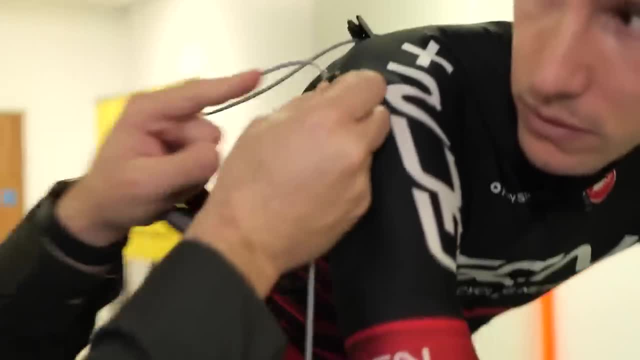 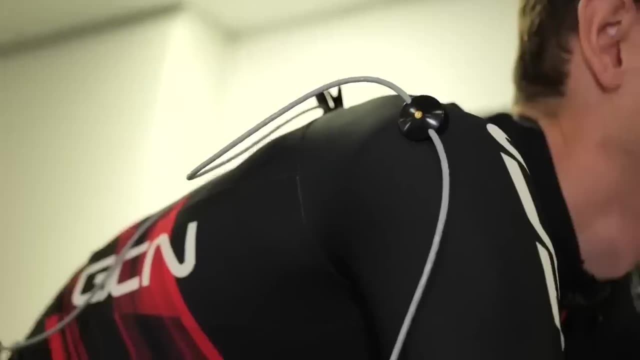 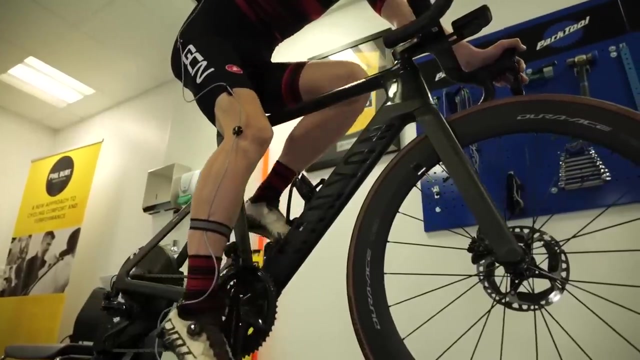 technology, your own experience, hands-on feeling where the joints are on people's knees and hips and, obviously, your experience from seeing hundreds, thousands of different people? Yes, I guess, do you find it's really beneficial to have that specific data from pieces of measuring technology, like the sensors that can 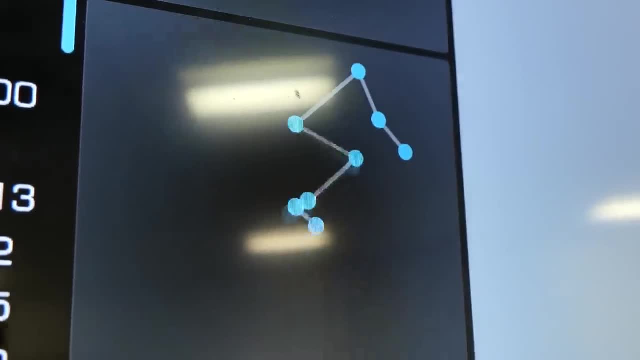 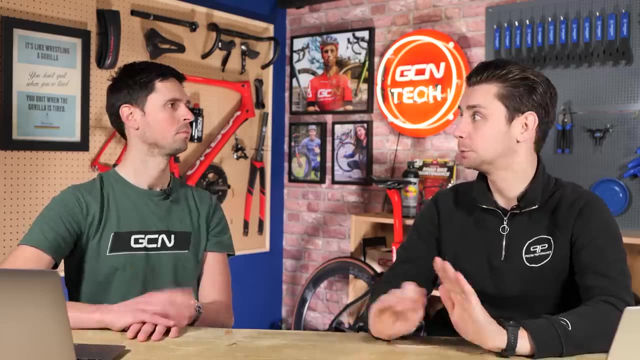 be put onto the body, I think when you're looking at very fine small changes. yes, definitely. I never personally rely on that system or that data capture 100%, because I feel like you have to call on your own experience and also the rider's. 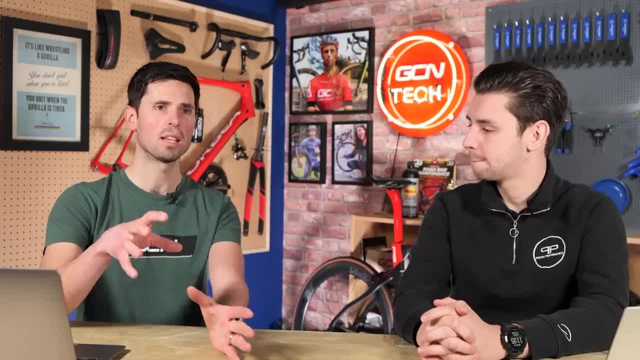 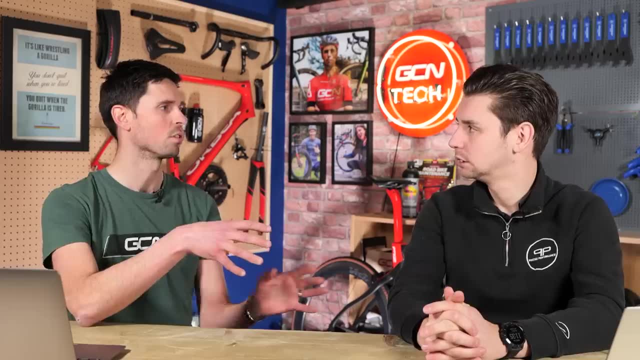 feedback. That's the most important thing. Do you think there's a way people could assess their crank lengths themselves at home without having to come and see someone with an in-depth knowledge on it? I would say probably not. Yes, Unless they are like you say, unless they. 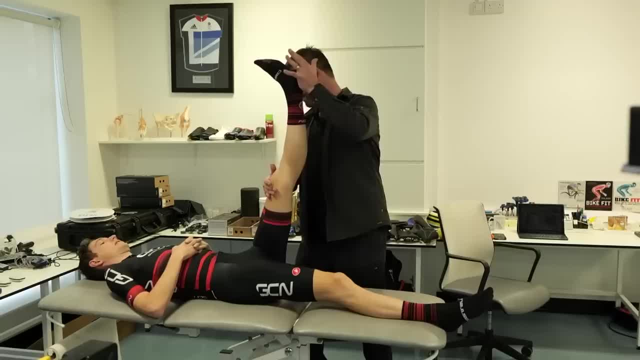 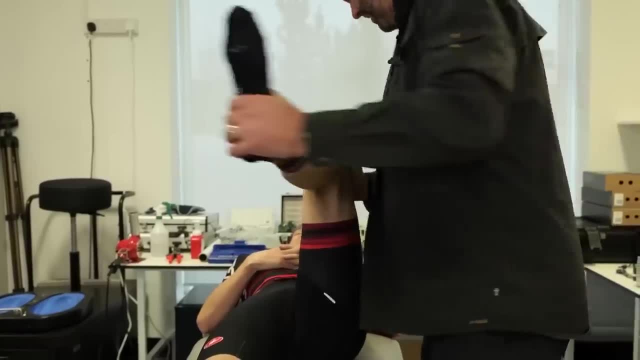 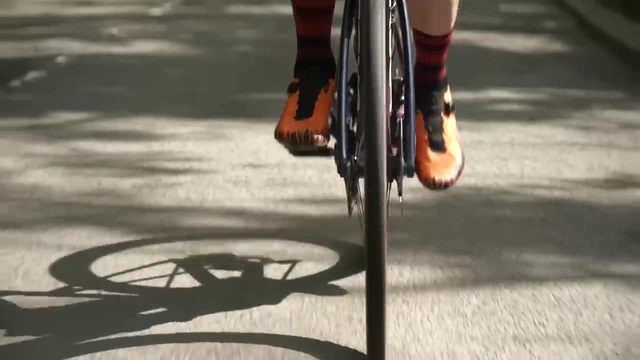 even know their body inside out? Yes, And know they have go simple hip impingement or hip limitations- Without seeing someone to say you have this imbalance or this impingement. they're probably not going to know they need to change their crank length. Personally, when I'm carrying out bike fits, yes, crank length is. 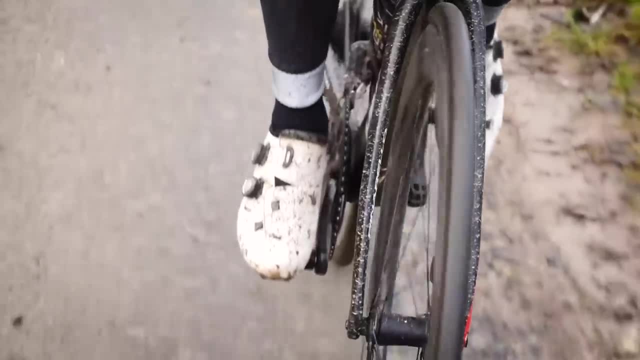 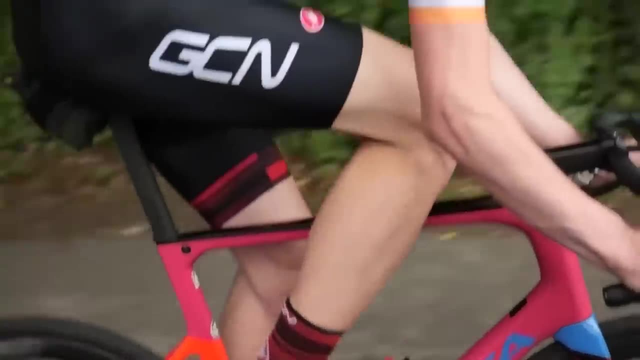 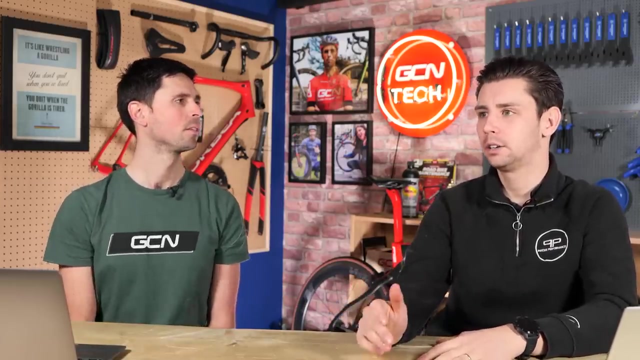 definitely on my radar. every bike fit, just to make sure we're not causing any issues to the rider. but we're also making sure that I don't recommend someone to go make an expensive change for no reason. In theory, there is a standard crank length that we see If you have, say, a 58 centimeter bike. 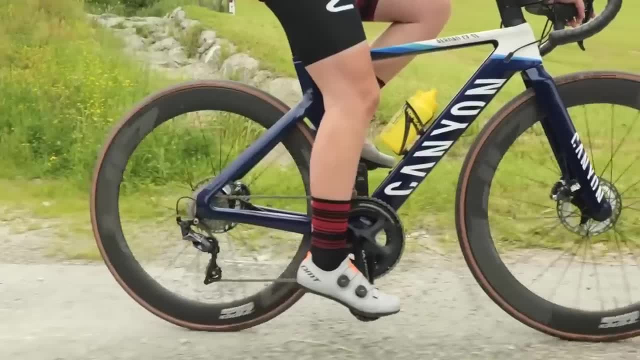 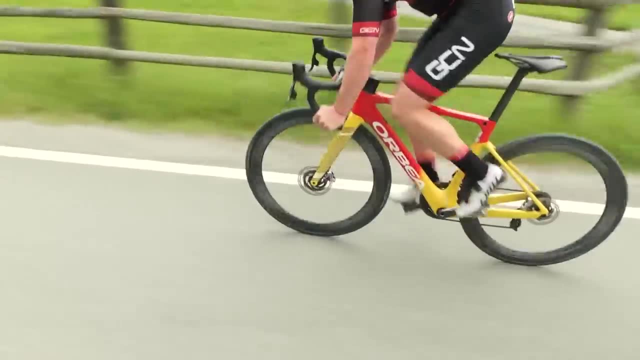 you're probably going to see a 175 crank length. If you have someone on a 56, 54, they're probably going to be 172.5.. I'm not entirely sure where these standards have come from, but that is generally what you're going to see on the bikes. Is there a way that you think changing your? 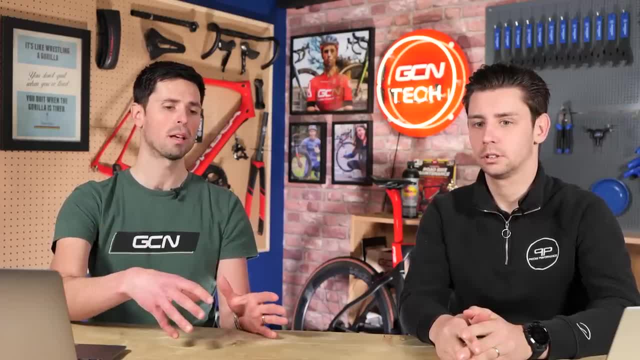 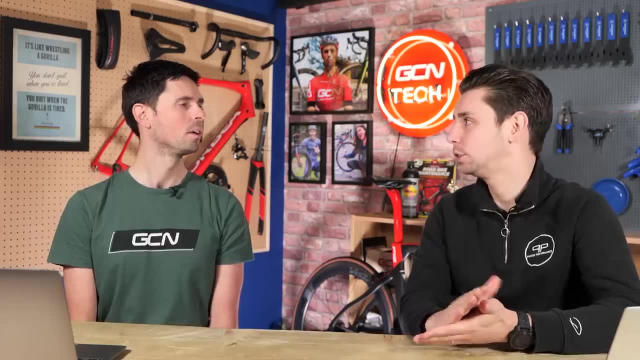 cranks can alter how you can position your body on the bike for a performance and aero benefit Absolutely. If you're running a shorter crank, you can lower your back angle, which then can ultimately lower your frontal area as well, all in tune with actually keeping the hip open as well. 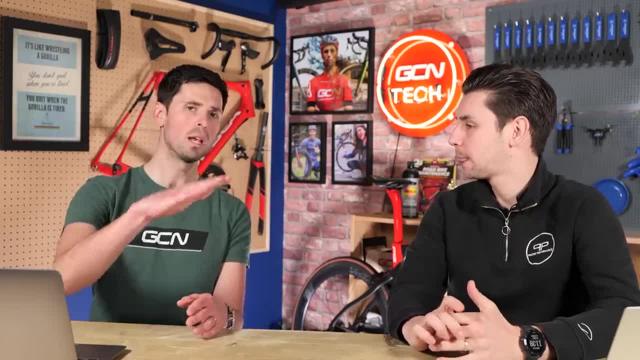 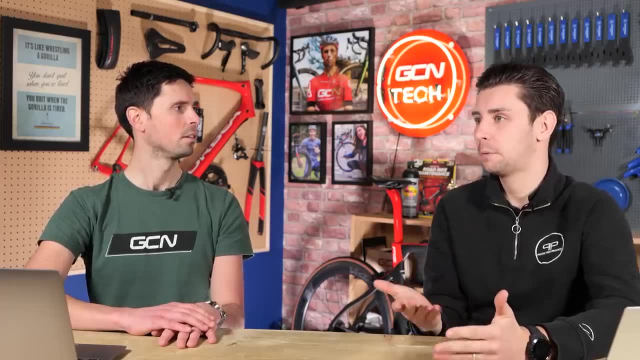 What's the theory behind that? You're saying you can lower your back angle. Is that purely on the basis of your knee isn't going to be coming up so high? Yes, Basically, your flexion of your knee isn't coming up as high, so you're not. 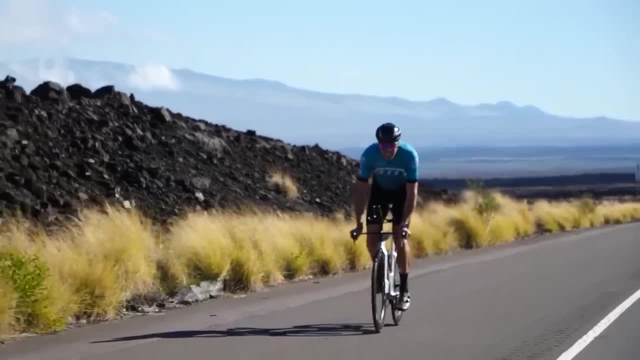 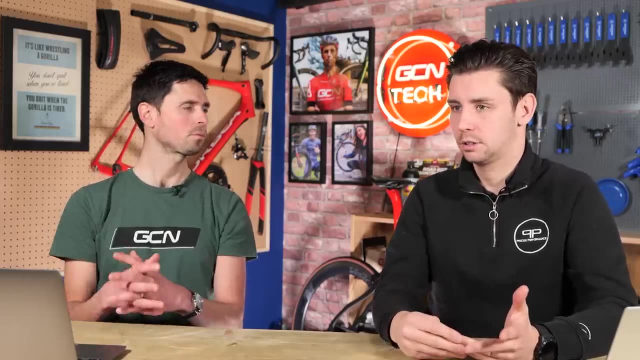 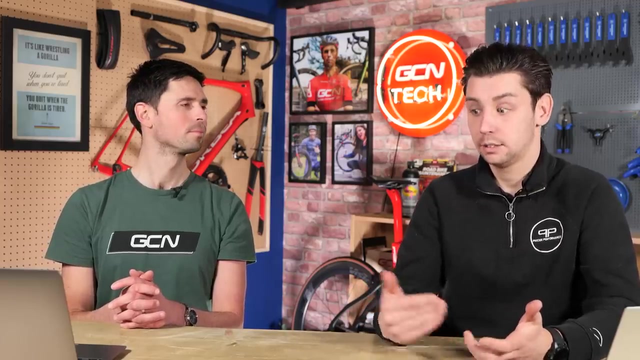 restricting your body as much. I think it's big in and more necessary in triathlon and TT, because people- Yes- are looking for that aero advantage. With the research and stats out there that we have, this is definitely a big shift of how people are riding, so making this change is definitely 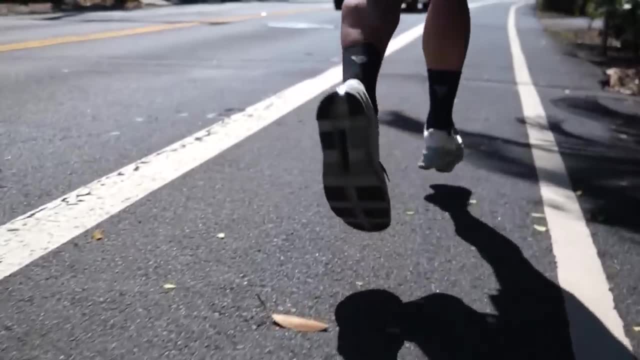 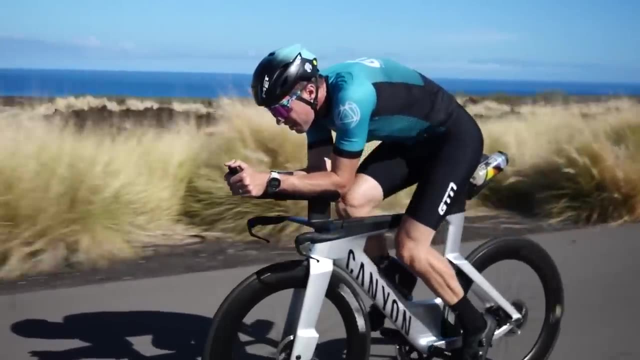 increasing performance. Sometimes a shorter crank for triathletes is purely just so they can run off the bike efficiently, Especially if you're doing a full Ironman- you've got 180k, especially if you're doing a flat course. you might be in that aero position for five hours, six hours. 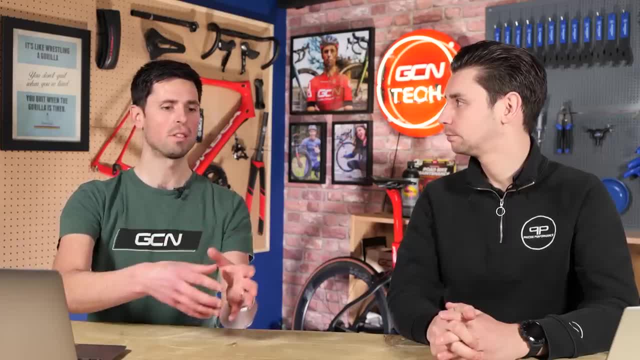 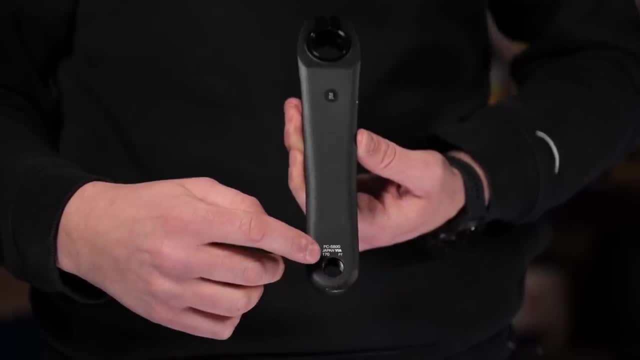 Give me a ballpark figure. Are we saying a 170?? Are we saying: find some more extreme crank length options? I generally hover around a 165, 170 range. That is quite short, isn't it for what typically people would see on their road bikes? Yes. Is there a reason why we can't just go shorter and shorter with cranks? It can cause you to struggle to get on top of that gear a little bit too much if you go too short. We have to keep that in consideration. This differs for everyone, so there isn't a black and white rule that is. 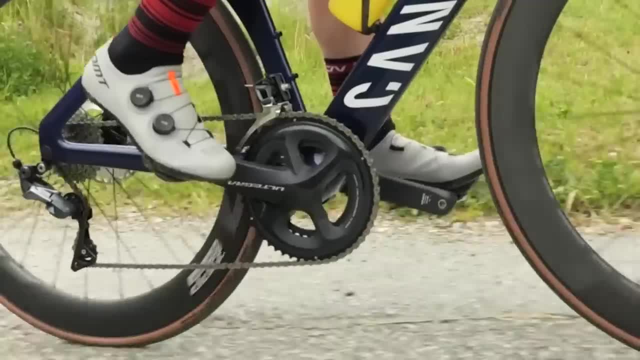 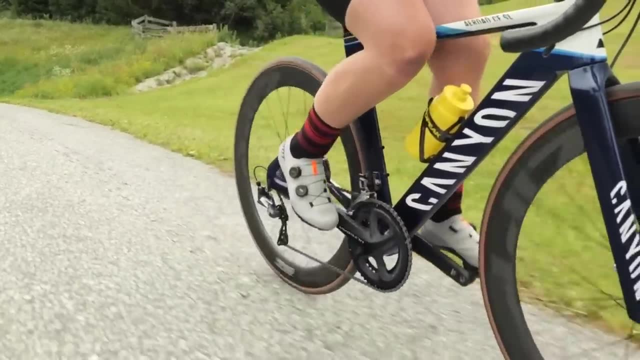 definite as such Shorter cranks. you need to make sure you've got appropriate gearing in the system to, I guess, account for the fact you've got a shorter lever. Yes, exactly, Okay, I'm going to get kitted up. You maybe just, I don't know, put your feet up. 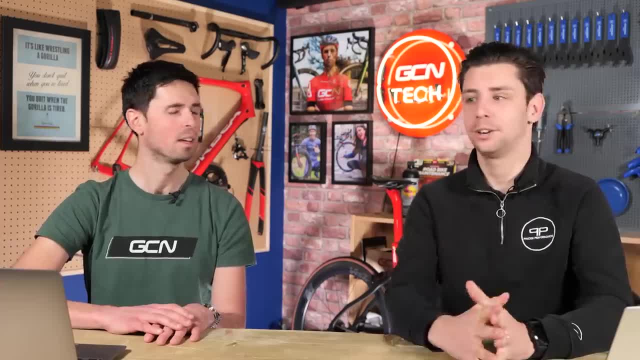 have a coffee tea. I'm going to have coffee. yes, That's free tea and coffee. Oh, definitely having a coffee then. All right, See you in a minute. See you in a minute, Okay, Thank you so much for the tea and coffee. I'm glad you enjoyed it, Are you? 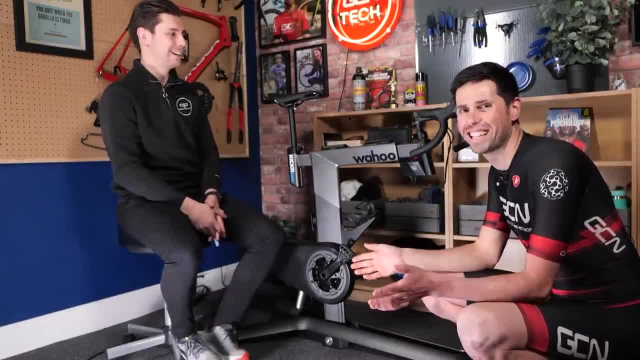 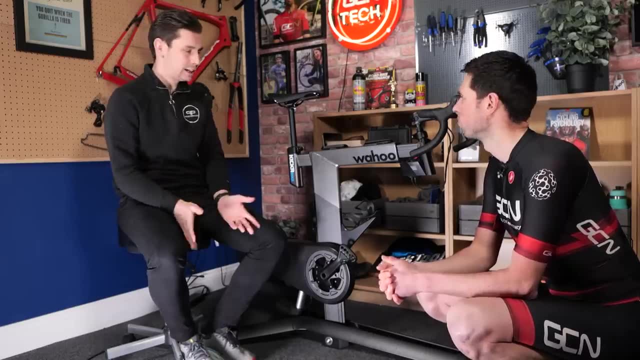 leaving money on the side. Yes, I'll do it later. Okay, Right. What's going on here, then? What I've done is I've taken your bike, grabbed the measurements off it, roughly transferred it onto this bike here, and I've noticed. 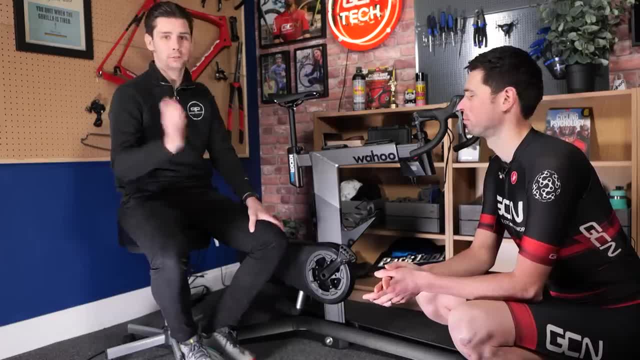 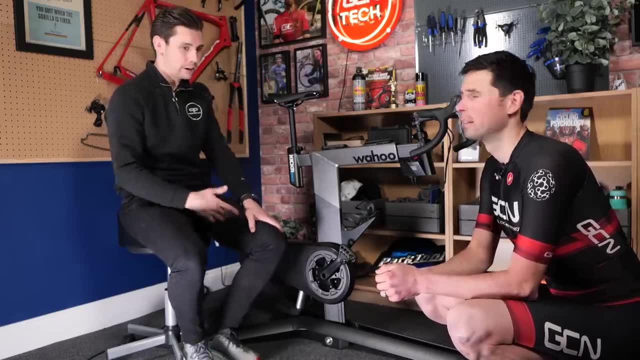 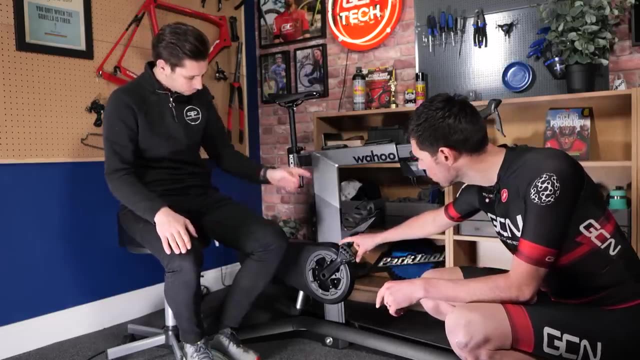 you ride 170 cranks on your bike. Correct Completely ignored it and I've gone for 175.. Fantastic, For the reason of trying to show yourself and everyone the difference between the extremes, like a 175 crank length to a 165 crank length. Is that the most we can do on these cranks? 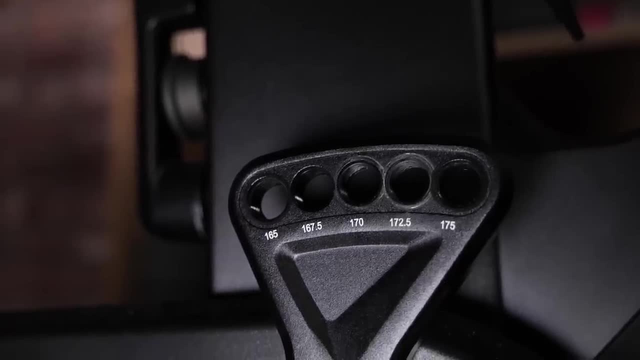 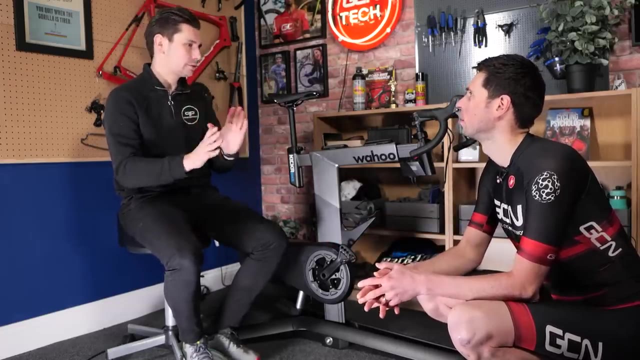 There's four different, no, five different ones here. Yes, there's five different options on this crank. here We're only going to focus on the two extremes. Yes, purely because it'll be easier to show the differences around it. Yes, 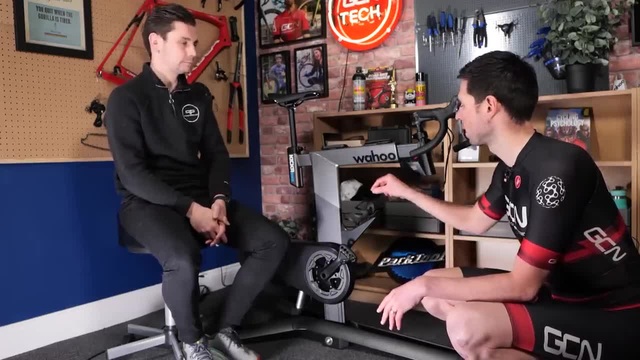 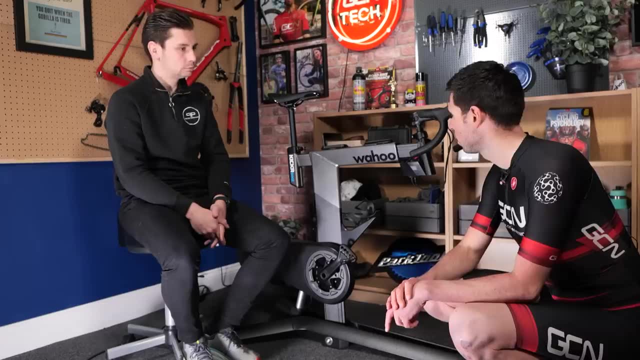 Well, we've already mentioned that the changes between one individual crank length is quite subtle and tricky to find. Hopefully, yes, this makes it super clear and visual. What's next? I guess I'd better get on the bike, should I? 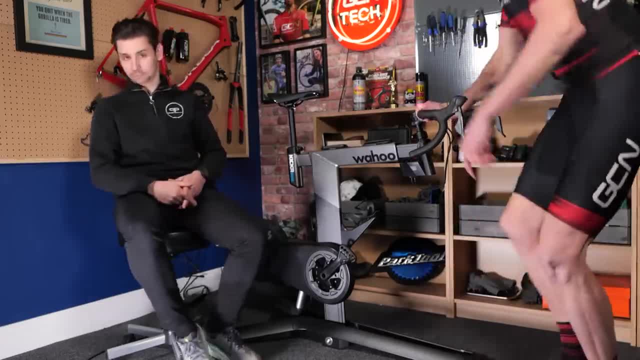 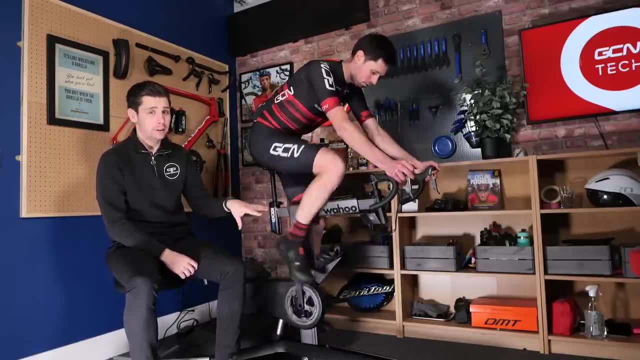 Yes, I think you'd better get on the bike and get some pedaling done Right. Let's do it, Alex, if you start riding for me. Alex is currently riding with the 175 crank length, which, in theory, closes his hip angle a lot more than he would do when he rides a 165. 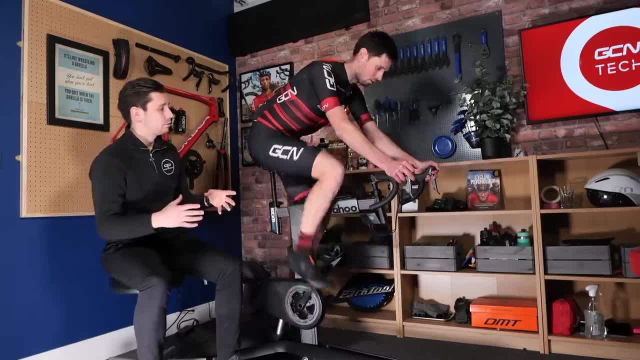 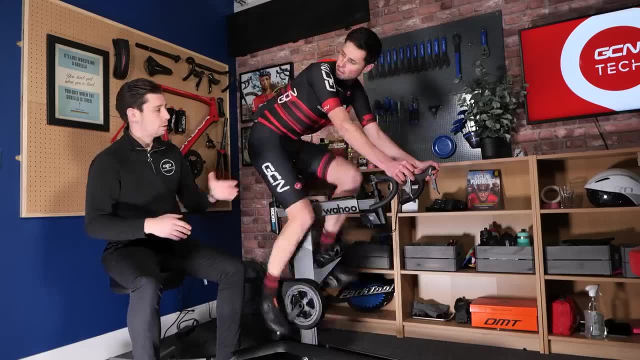 shortly. Yes, There's a few different positions that you can ride in and we can monitor how much your hip angle can close, whether that rider is riding on the hoods, like Alex is now, or whether, if you want to change to the drops, To the drops, so it brings my 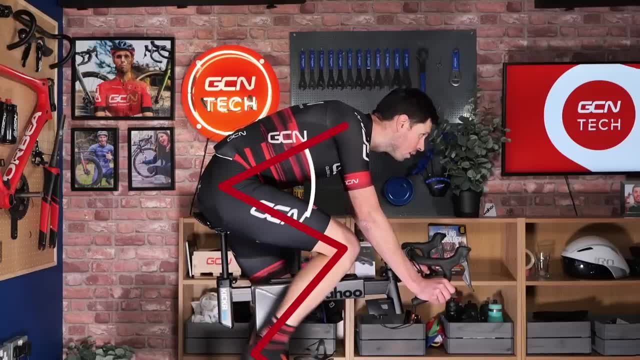 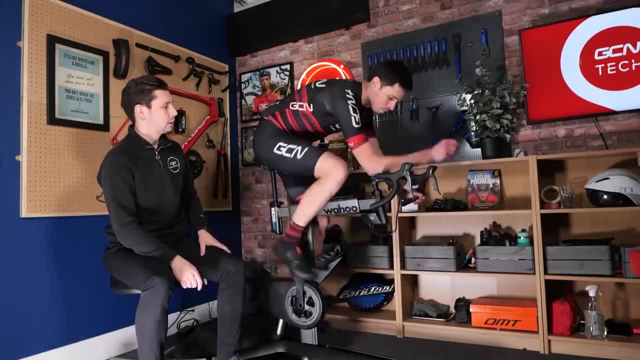 chest lower to the handlebars, Exactly, and we can see how the hip angle is closed. again, If we look at a really extreme position, maybe like on a TT position, I can just rest my arms on the bars. I guess sort of like this You can feel- 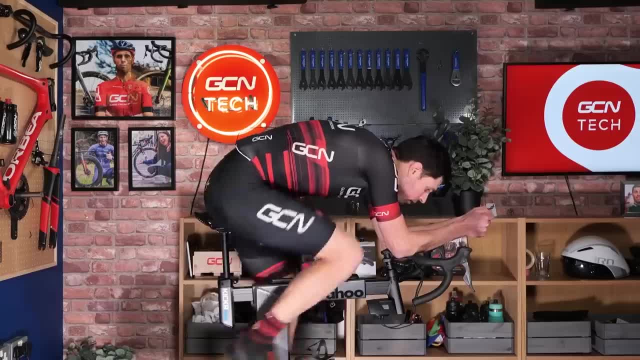 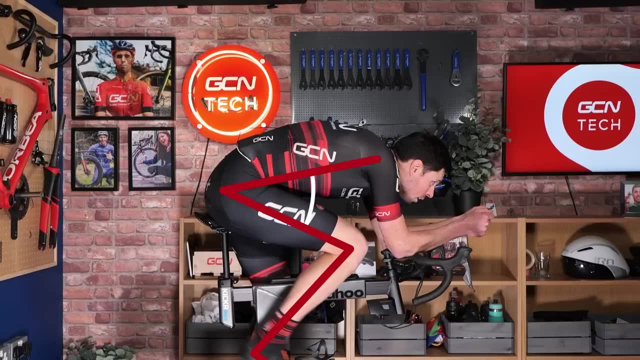 You might get the UCI after you on that one, though. Yes, I can feel the difference of how much it's- It's really coming up towards my chest, my knees and thigh. Yes, This is probably the most visual difference we're going to see in terms of how much this 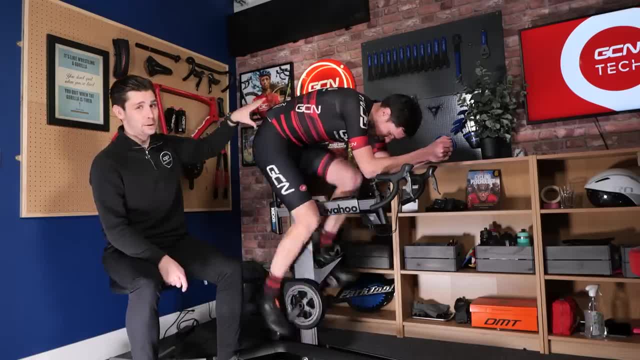 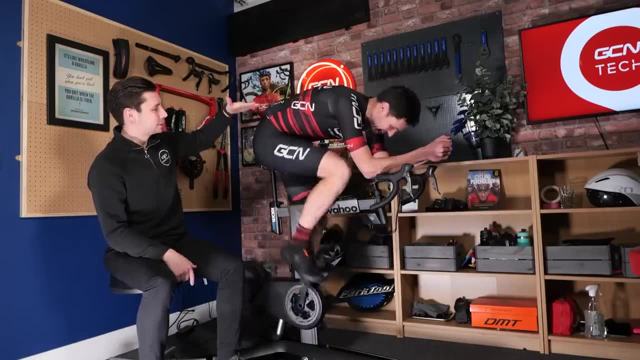 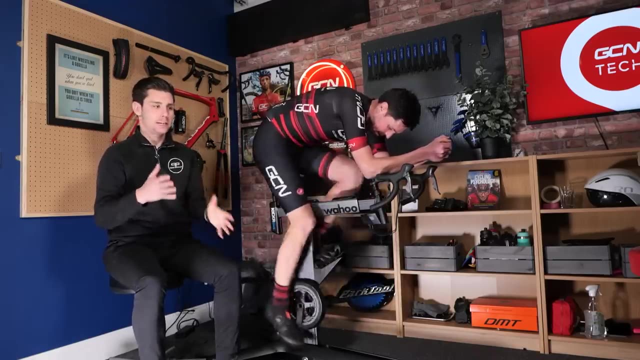 hip angle is closed. Now we know that Alex's hips don't have any limitations or impingements. Oh, these hips don't lie, Jake, They do not. We're not seeing any adverse pedaling alignment or any hip kickback in terms of the knee wanting to pop out at the top of the pedal stroke. 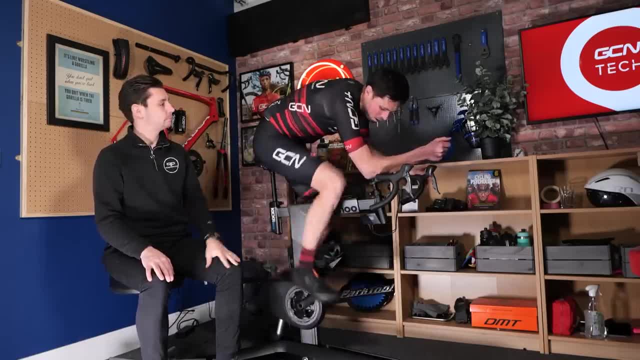 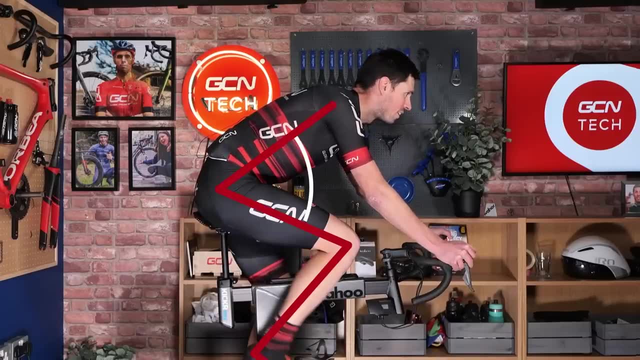 but we can see that visual closure of the hip. It is noticeable. I know that you've just told me they're 175 cranks, but I do feel like, because there's a bigger jump from what I normally ride, I can tell the difference. on that. Shall we change the position of these cranks? 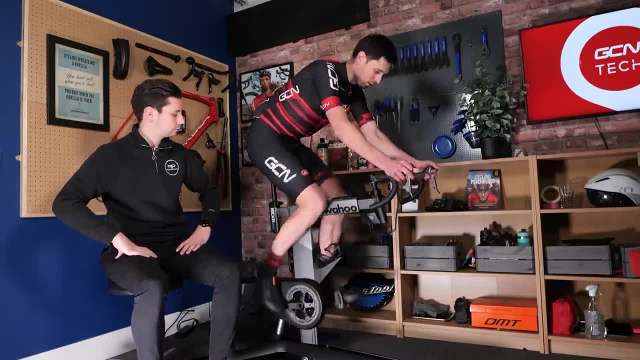 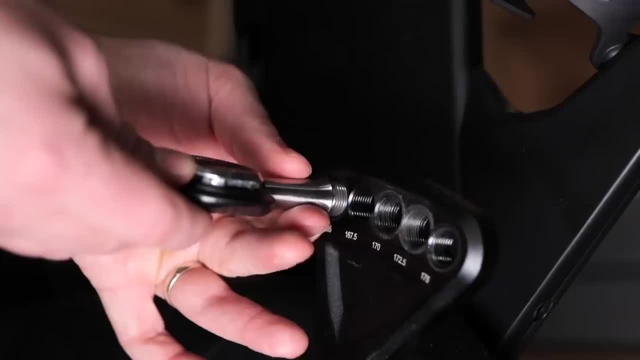 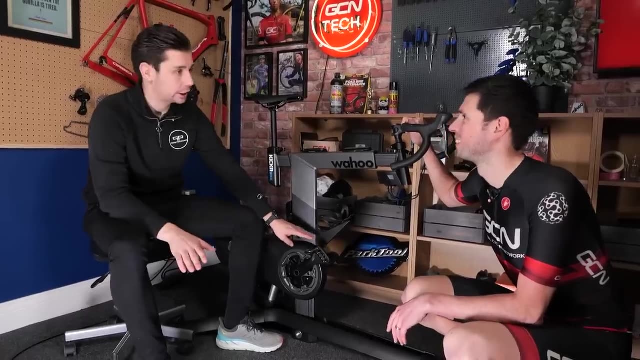 Yes, Change cranks and then we'll see the differences. I'll do the hard work. You sit there, Don't worry. Can I have another coffee? Yes, 165 long. Okay, Way easier than changing the chain set. Yes, 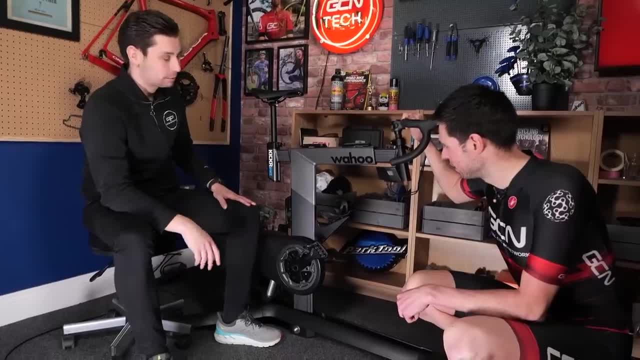 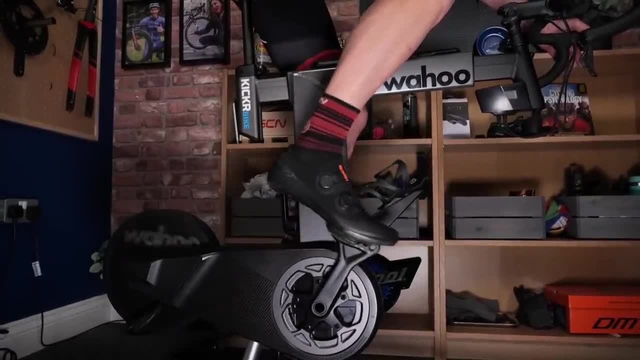 Let's get you on the bike and we can see how you feel with riding with a shorter crank. now, All right, You sit down, I'll do the hard work. Thank you very much. Lovely, Even just as I'm getting started pedaling now already. 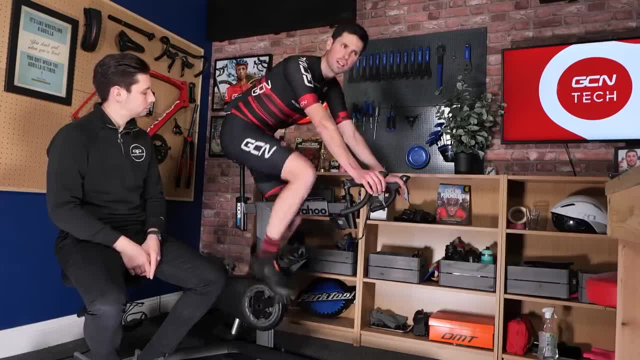 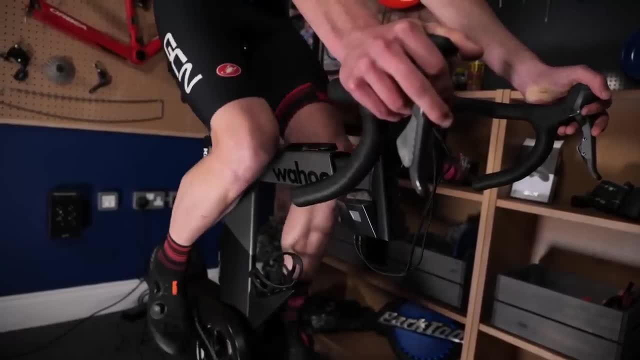 I can instantly tell there's a huge change in my cranks. It's almost leading me to say that it feels like my saddle's now too low. Yes, I think that's a pretty valid point. When we do a big change like 10 mil, that could definitely warrant a saddle height change. 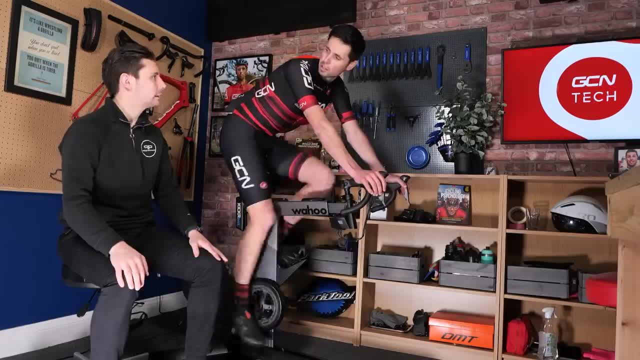 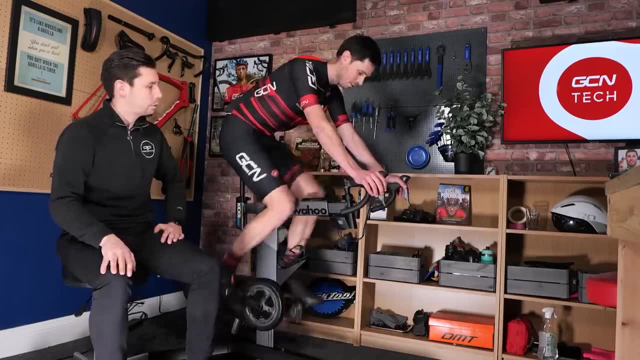 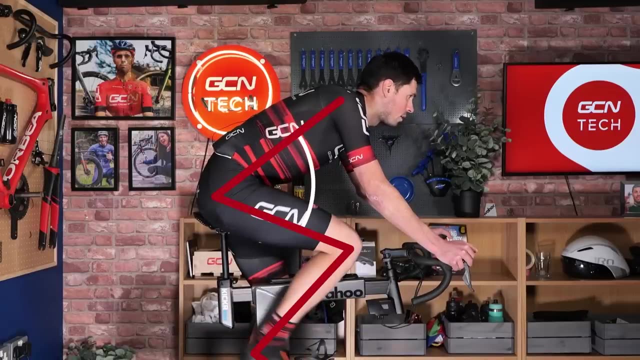 maybe just a 5 mil or around that sort of To compensate for the change, To compensate the change, exactly. Okay, What are some of the differences that we can see from this cranking? now, When we compare the difference between the 175 crank and the 165 crank, we can really see how the hip is not being closed up as much. 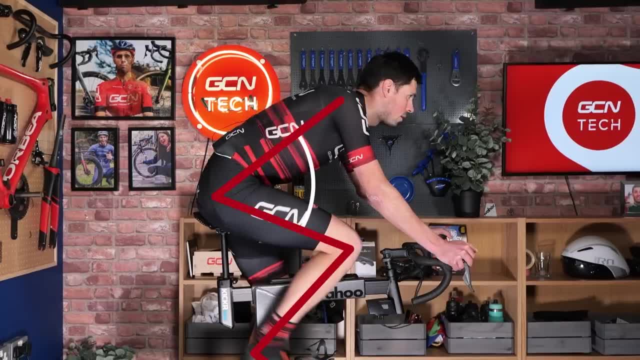 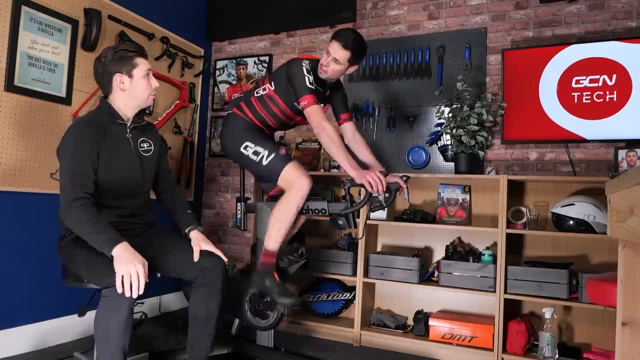 which, in theory, is just keeping the hip open, reducing your risk of injury, possibly allowing you to then come down a little bit lower in the front end of the bike, and allowing us to improve our efficiency for our pedal stroke. In fact, I'll ride on the drops now and I can already feel that. 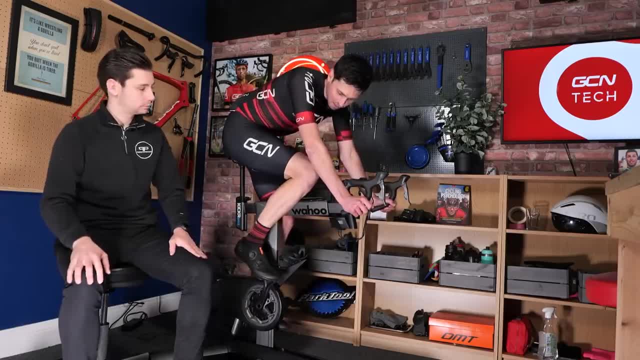 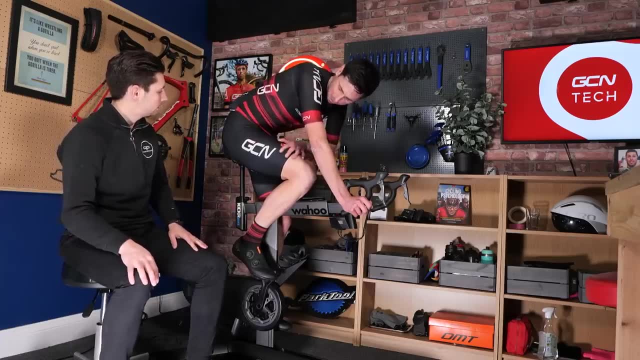 yeah, like you say, opening up the hip angle, which I guess, if I stop my leg towards the top of the pedal stroke roughly there. we're talking about this difference here. so this angle of my hip to my thigh relative to my torso, Is that right? 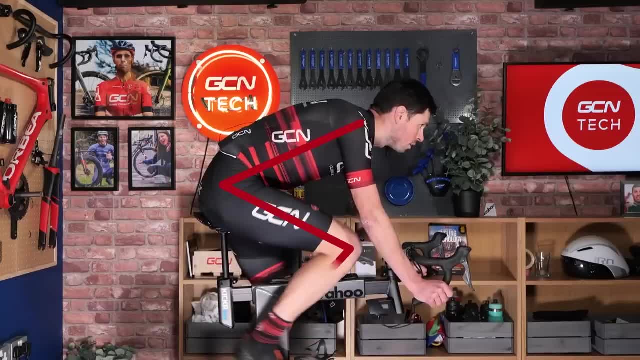 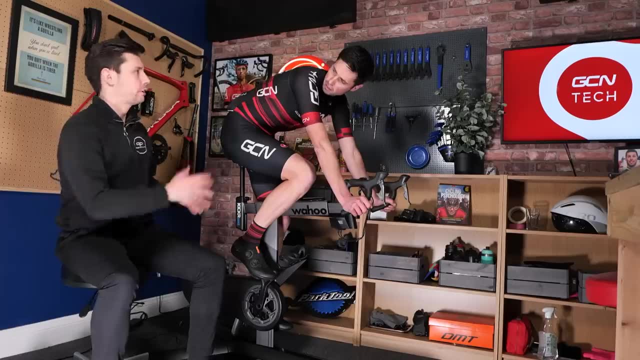 Exactly yes, From the torso to the hip and coming down the femur. here, Sometimes the easiest place to see it is the gap in between the stomach and the top of the thigh. just from a reference point, rather than trying to get into the nitty-gritty angles as such. 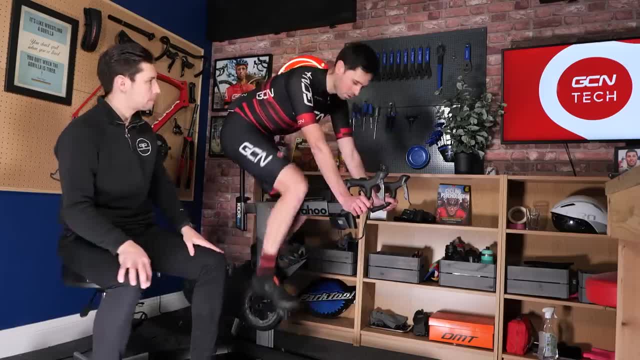 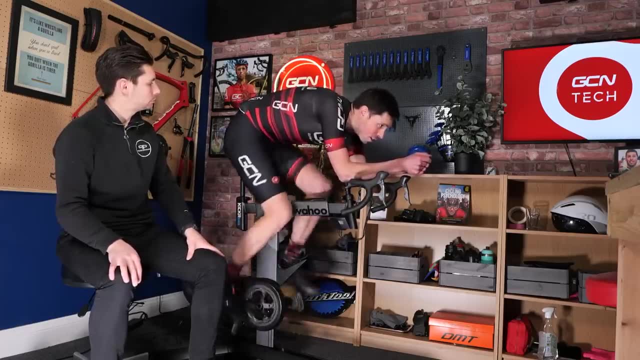 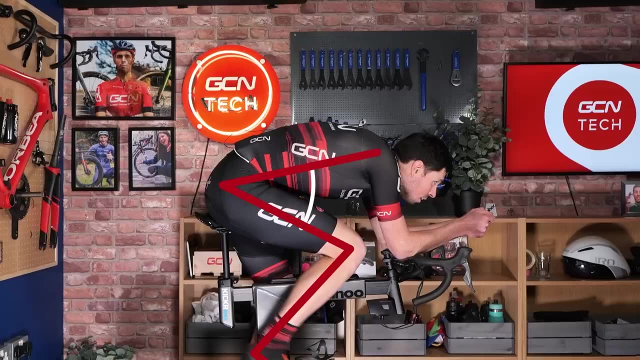 Then when we have the longer crank set in, I also rode in a more extreme time trial-esque type position. If I do that now, I can again feel the difference that just quite simply, my knees aren't coming up as high. No, exactly. Again, that gap is obviously closed more from when the two previous positions were. 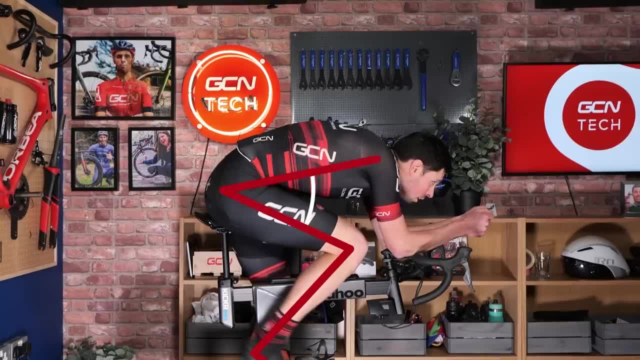 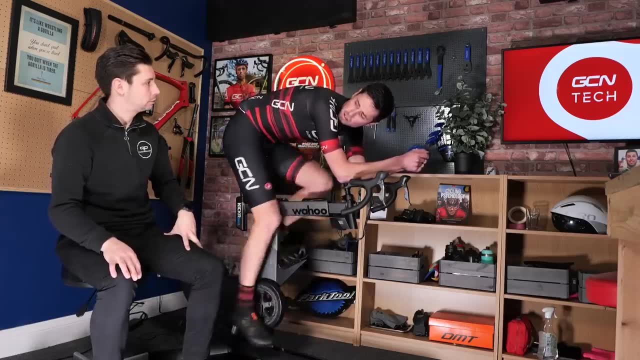 but in comparison to the 175, again, it's definitely a lot more open. You can see how it does impact people that are doing time trials and triathlon in such a huge way, because you'd never ride like this on a road bike. 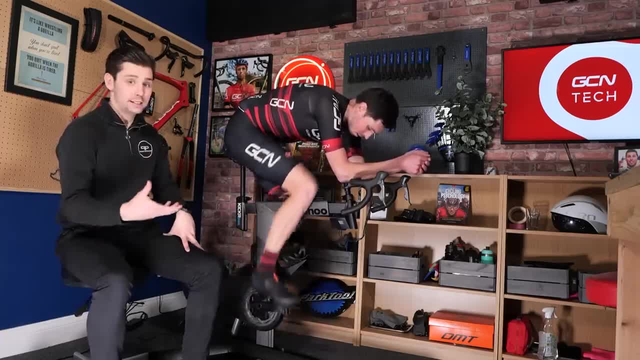 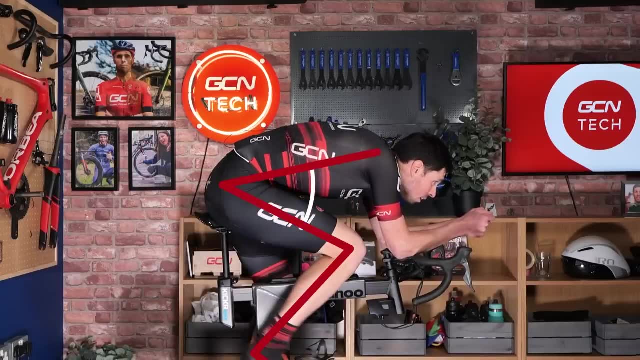 No, No, exactly not On a TT triathlon scenario. you're going to end up having a lower frontal area, which is going to allow you to be more aerodynamic and plus, like I said earlier about being able to run off the bike. That's really interesting to not only. 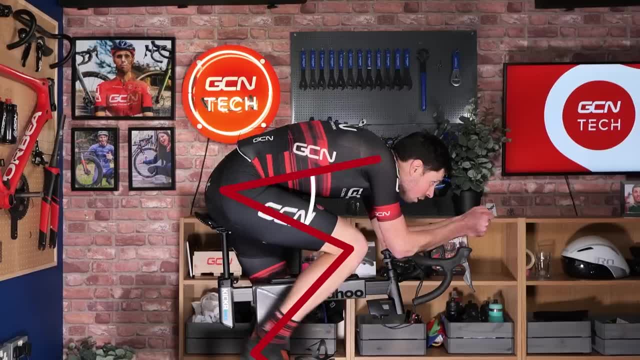 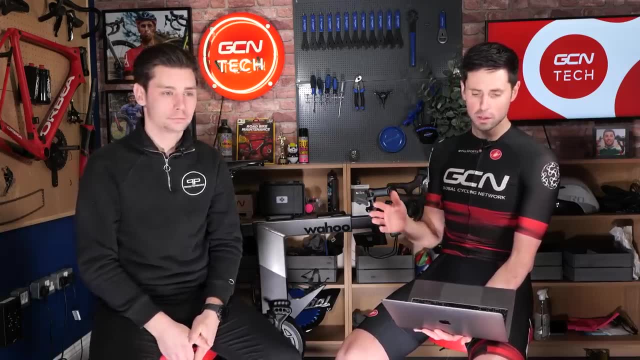 experience that experience. That's an extreme difference myself, but be able to clearly visualize it for everyone at home. Before we wrap this thing up, I've got a couple of quickfire questions I want to throw at you. Do you think everybody should be looking at, changing or investigating into their 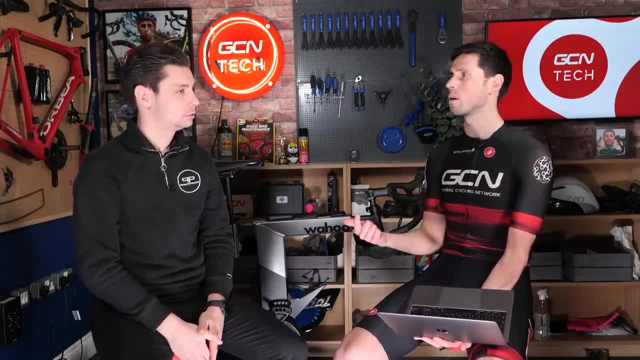 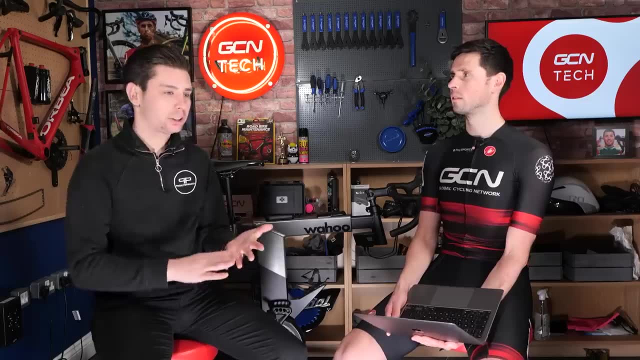 crank lengths, firstly for beginners and then for more experienced riders. I was going to say it's a bit of a two-answer question really, If you're new to cycling recreational and you're not experiencing any issues or pains or injuries. 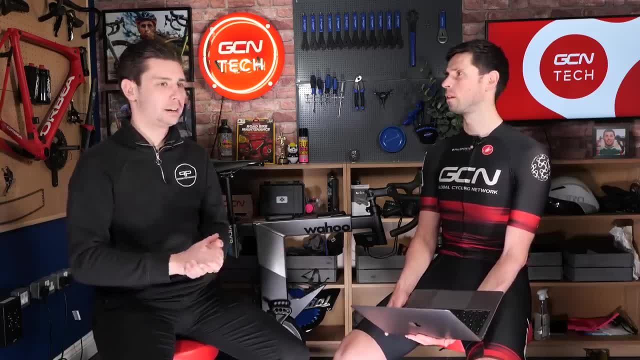 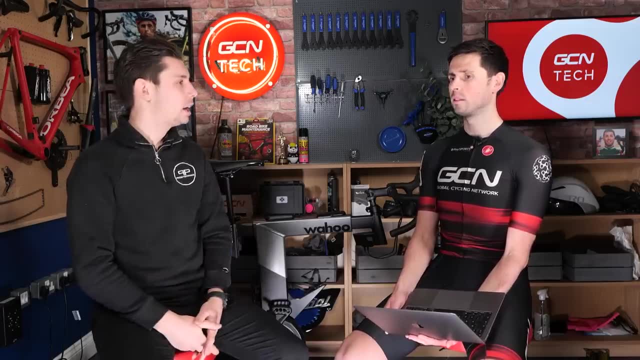 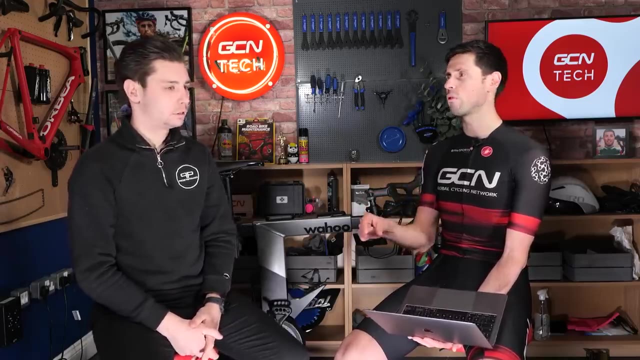 potentially, we don't need to disrupt that area for that person. If you're trying to find those marginal gains, maybe it's something you might want to investigate in. Potentially, if you are feeling some pains as well, then that's something we should look at. That's very helpful. Does altering our 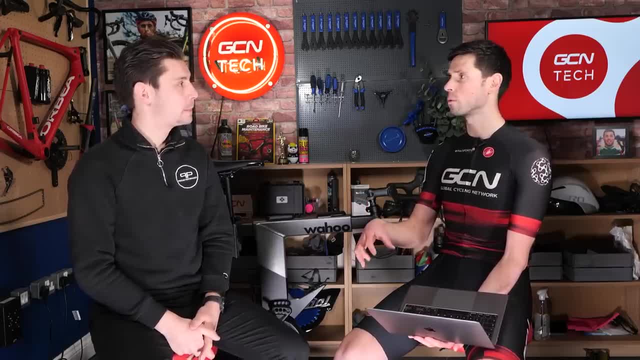 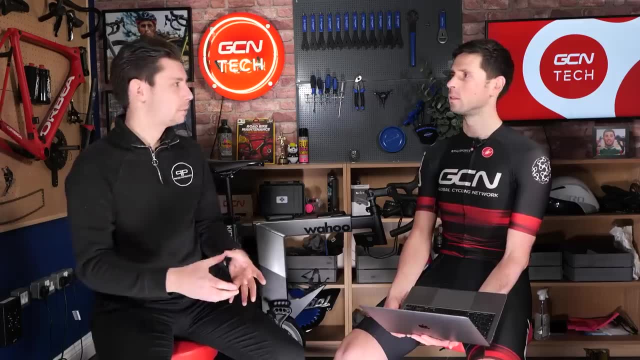 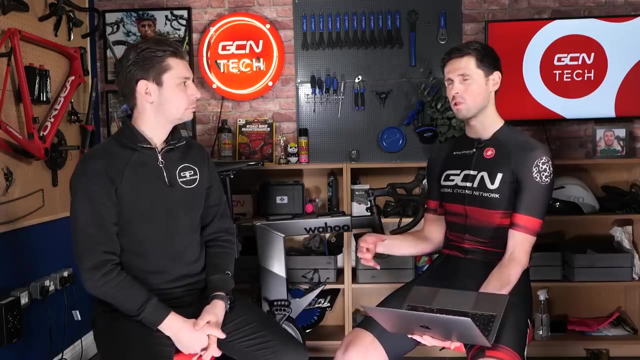 crank length, change the muscle groups that we're using? In theory, no, because if the bike is set up properly, we should still be recruiting the same muscles to ride efficiently and the bike power. That's interesting. I was assuming that it might have changed it, but no, fair enough. 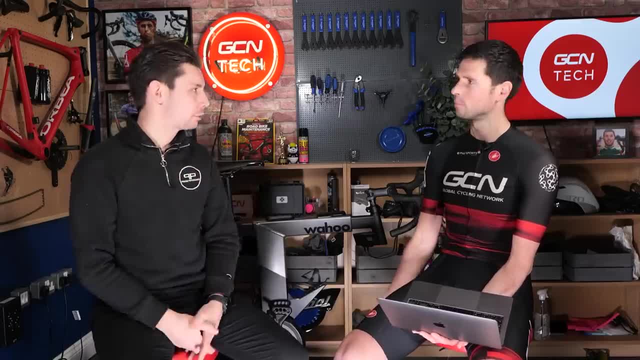 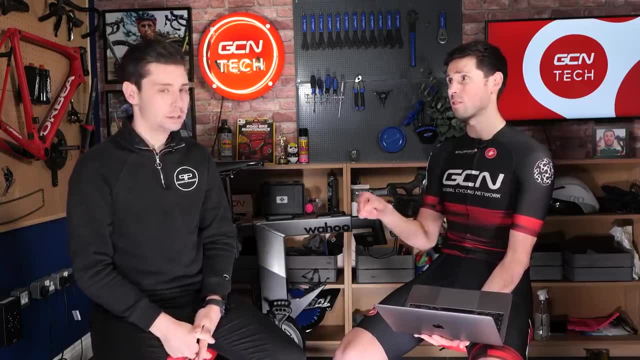 There could be subtle differences, but in theory the same muscles are going to be recruited In a few weeks' time. actually, I'm doing the track national challenge. I'm going to race the individual pursuit Now, Oli tells me. 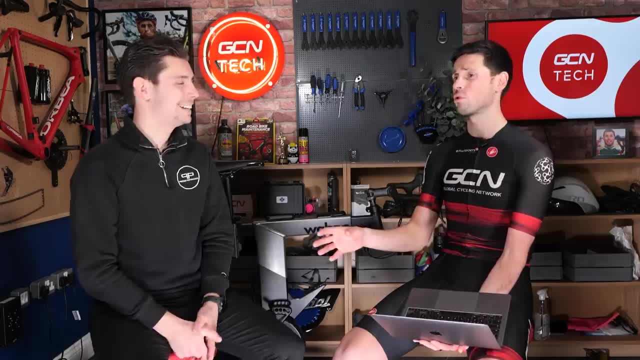 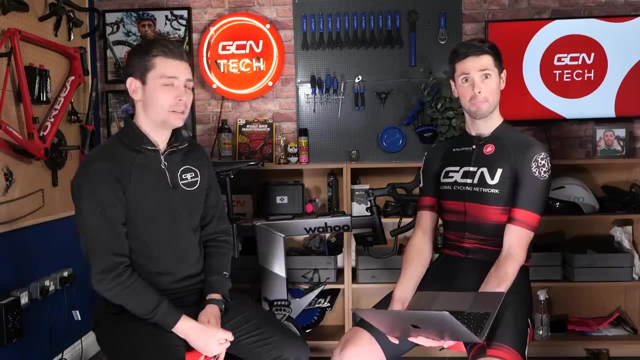 I've got to use short cranks. He's like it's going to revolutionize your cycling. use short cranks. Is he right, and is it something I should investigate further into? Yes, I do agree with Oli. Yes, you should definitely investigate that. 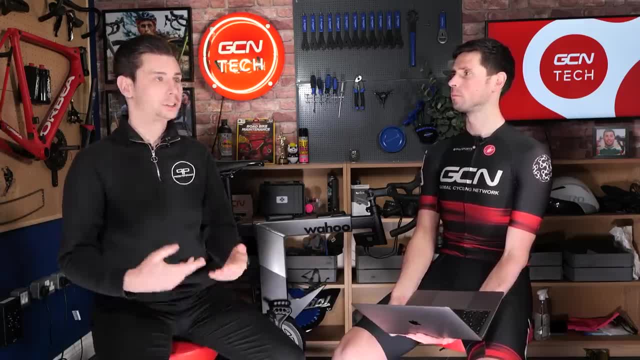 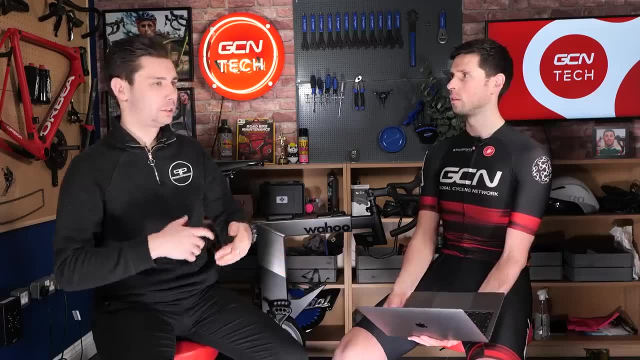 I think, going back to some of the points you made, you can potentially look at improving your frontal area for aerodynamic gain, but obviously as well keep an eye on your gear ratio, making sure that you can actually ride efficiently and don't come into any problems from going too short. 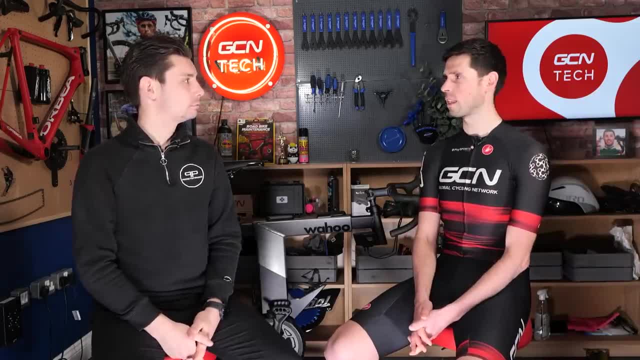 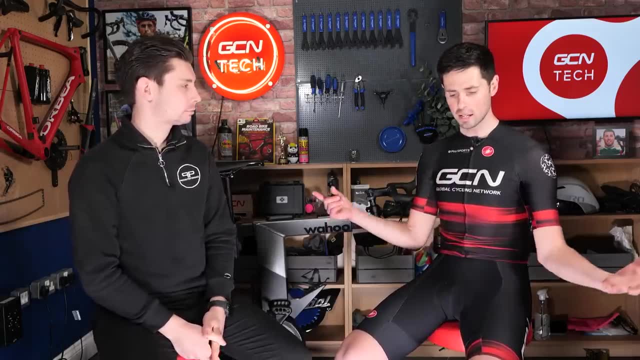 All right. All I guess I need to say is thanks for coming down and talking through crank length with us. I found it really interesting. I hope everyone at home has found it interesting as well. What's our main takeaway message from this? The main takeaway message from: 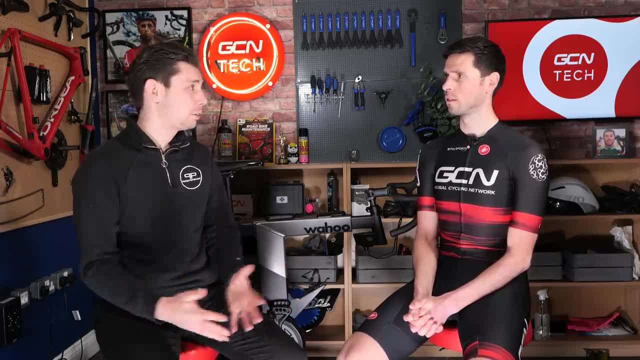 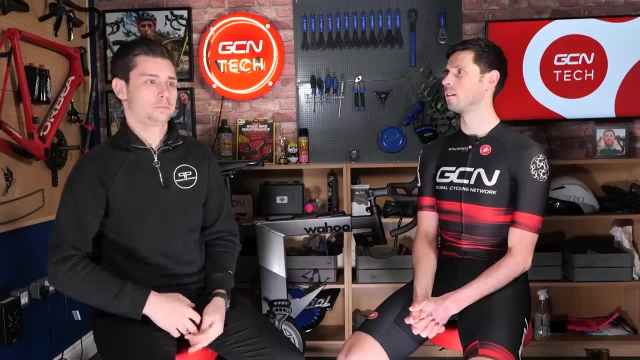 this is, if you don't really have any issues, maybe don't go searching to find an issue or solve an issue. If it's not broken, don't fix it. If you are looking for those marginal gains, looking to make a little bit of improvement to your performance, potentially it's something.